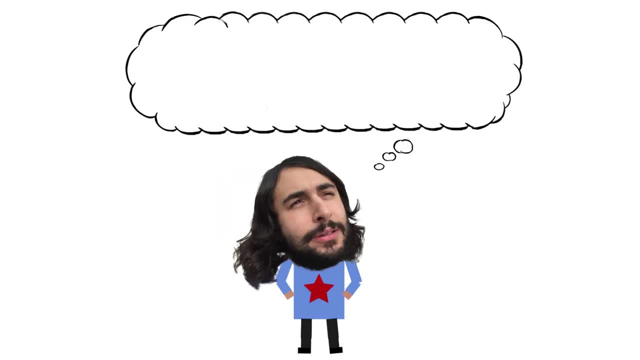 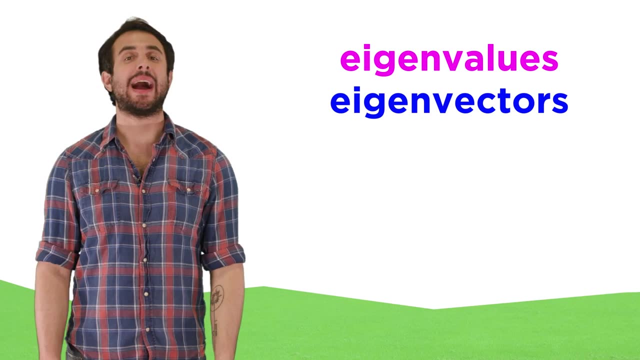 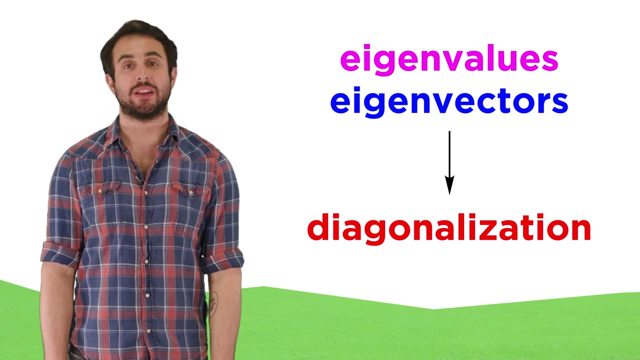 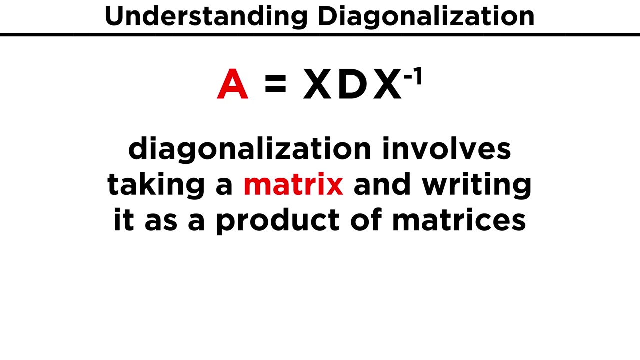 Professor Dave, again, let's get diagonal. Now that we have learned about eigenvalues and eigenvectors, it's time to learn about their applications. So let's start by learning about something called diagonalization. Diagonalization involves taking a matrix and writing it as a product of matrices. one of 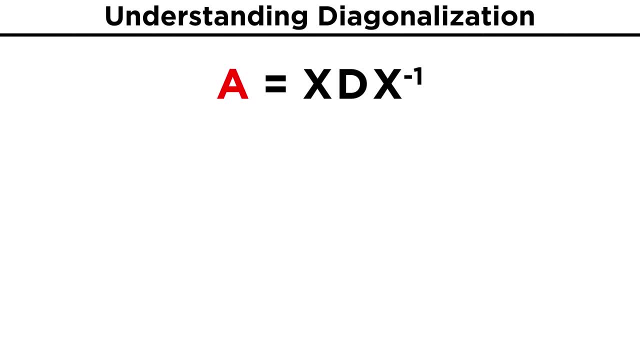 which only has values along the diagonal. For example, if we have matrix A, we will write it as X, D, X inverse, where D is a diagonal matrix. If we move the X matrices to the other side, we see that X inverse AX equals D, The X. 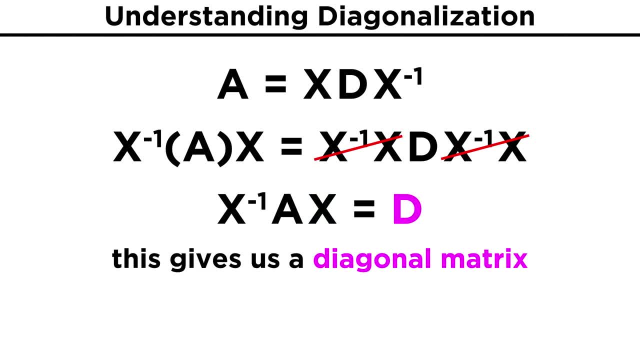 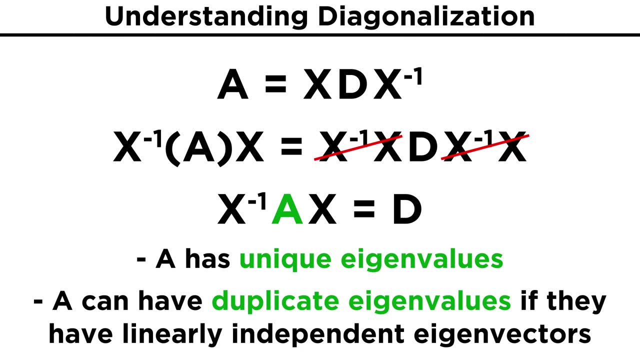 matrix is said to diagonalize A, because multiplying A in this way gives us the diagonal matrix D. This process only works for matrices that have unique eigenvalues, or if there are duplicate eigenvalues, then there must exist linearly independent eigenvectors for the duplicate. 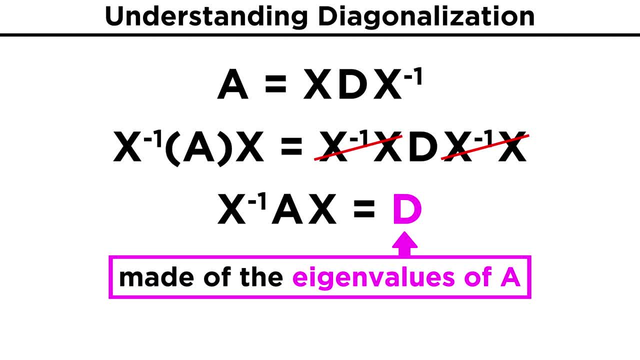 values. The reason for this is that the diagonal matrix D is simply made up of the eigenvalues of A, while the matrix X is made up of the eigenvectors. So, fortunately, once we know the eigenvalues and eigenvectors of a matrix, the diagonalization. 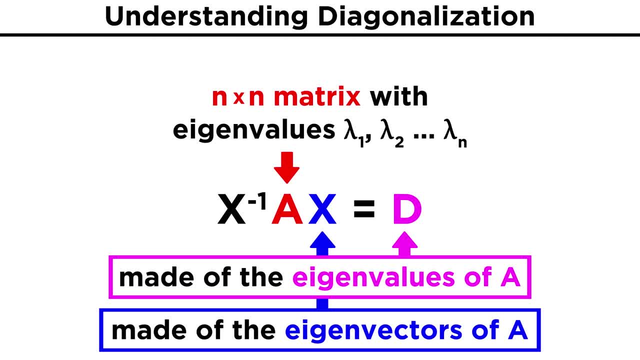 process is easy. Let's assume an n by n matrix A, which has eigenvalues lambda one, lambda two to lambda n. Then the diagonal matrix D is just those eigenvalues placed along the diagonal, with zeros for all the off-diagonal elements. 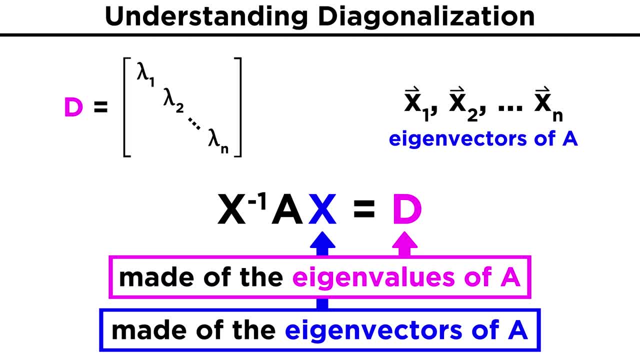 Now, if X1, X2, to Xn are the eigenvectors for those eigenvalues, the matrix X will have columns made up of those vectors In the same order as the eigenvalues going down the diagonal, such as X1, X2, to Xn. 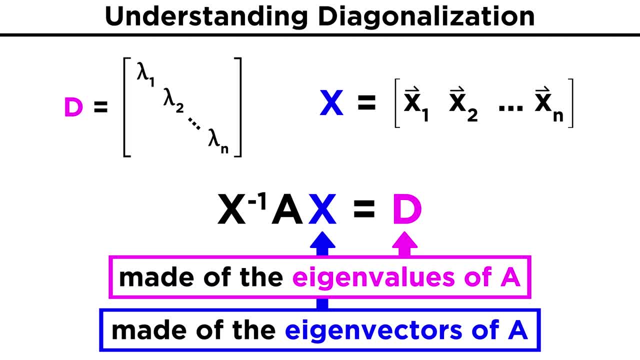 It's important to note that, while we can place the eigenvalues and eigenvectors in any order we want, once we find them, we must remain consistent in how we order them in these matrices. The first column of the X matrix must be the eigenvector associated with the eigenvalue. 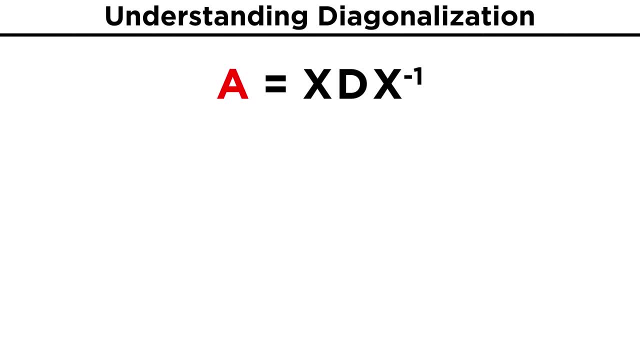 which only has values along the diagonal. For example, if we have matrix A, we will write it as X, D, X inverse, where D is a diagonal matrix. If we move the X matrices to the other side, we see that X inverse AX equals D, The X. 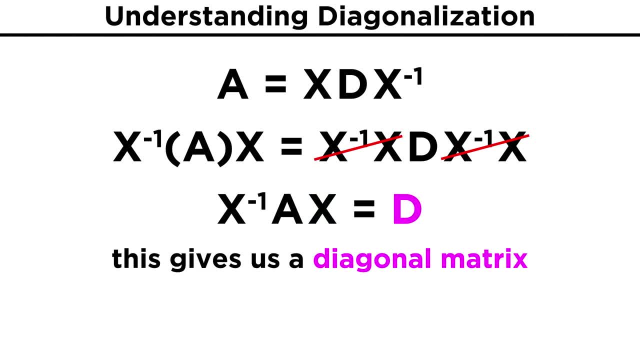 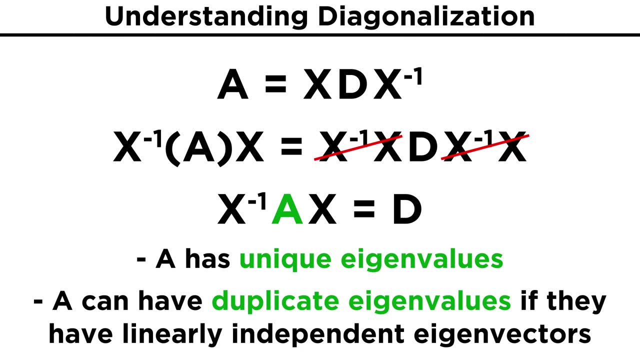 matrix is said to diagonalize A, because multiplying A in this way gives us the diagonal matrix D. This process only works for matrices that have unique eigenvalues, or if there are duplicate eigenvalues, then there must exist linearly independent eigenvectors for the duplicate. 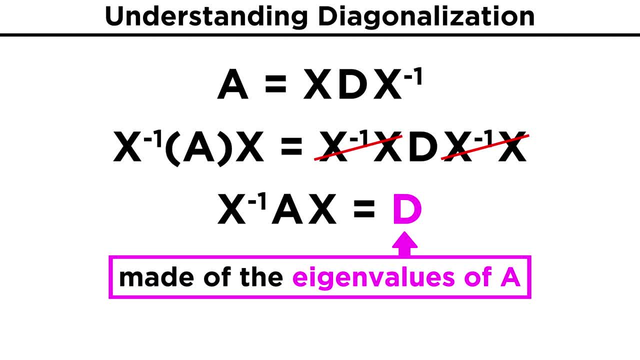 values. The reason for this is that the diagonal matrix D is simply made up of the eigenvalues of A, while the matrix X is made up of the eigenvectors. So, fortunately, once we know the eigenvalues and eigenvectors of a matrix, the diagonalization. 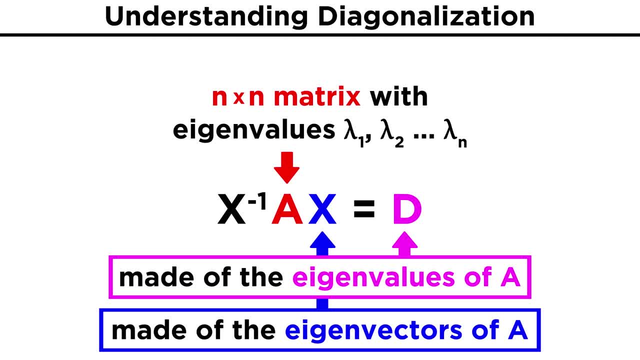 process is easy. Let's assume an n by n matrix A, which has eigenvalues lambda one, lambda two to lambda n. Then the diagonal matrix D is just those eigenvalues placed along the diagonal, with zeros for all the off-diagonal elements. 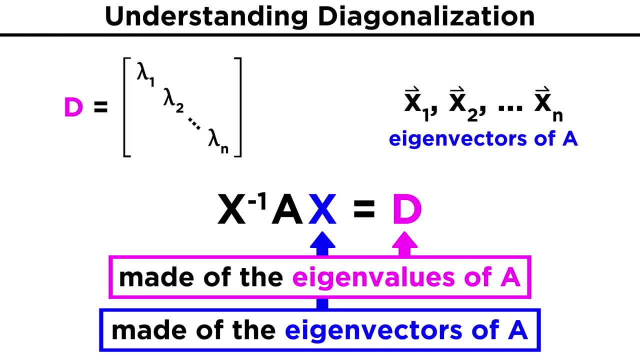 Now, if X1,, X2, to Xn are the eigenvectors for those eigenvalues, the matrix X will have columns made up of those vectors. So, for example, if we put the numbers of the eigenvalues and the vectors in the same order, 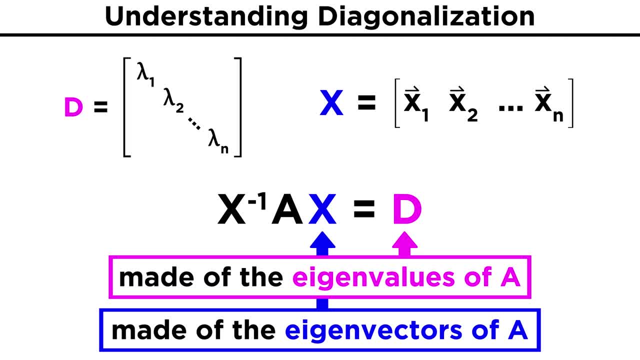 as the eigenvalues going down the diagonal X1, X2, to Xn. It's important to note that, while we can place the eigenvalues and eigenvectors in any order we want, once we find them, we must remain consistent in how we order them in. 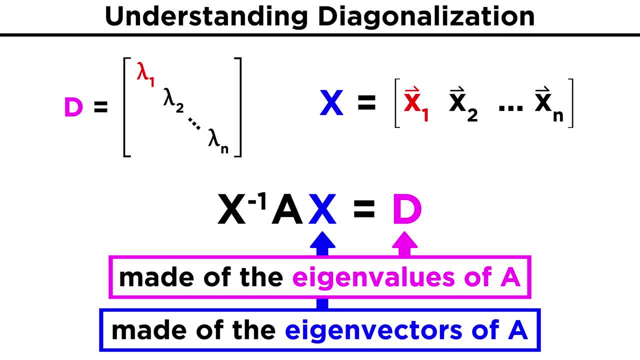 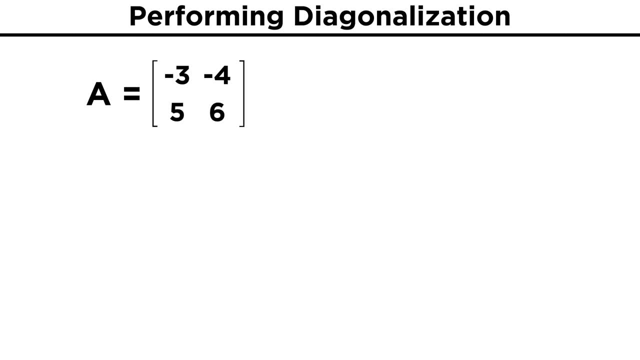 these matrices. The first column of the X matrix must be the eigenvector associated with the eigenvalue for the diagonal of D, Same with the second column of X and the second term for the diagonal of D, and so on. Let's look at an example. 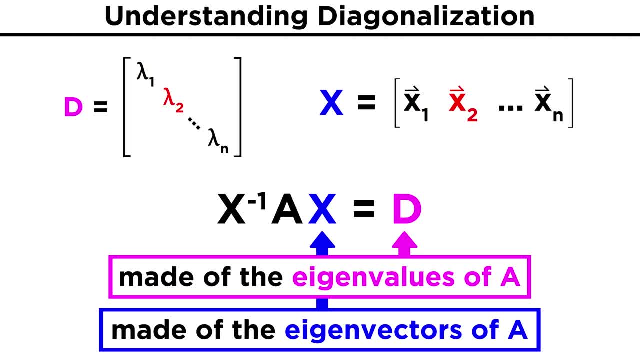 in the first term for the diagonal matrix. That's how we will solve it. Thank you for watching. I hope everyone had a nice day. Bye, bye, Bye, Bye, bye, Bye, bye. of D, Same with the second column of X and the second term for the diagonal of D, and. 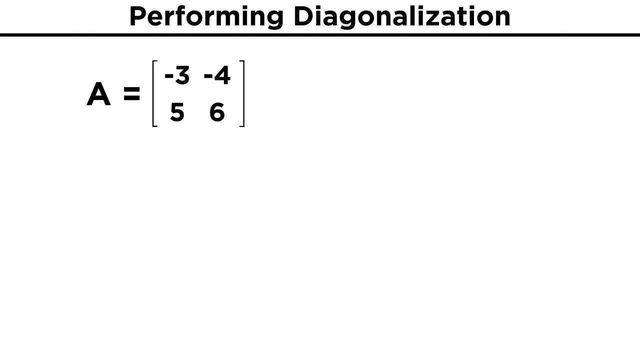 so on. Let's look at an example. Consider the matrix A, with entries negative three, negative four, five, six. We must first find the eigenvalues, which means we must solve for the values of lambda that satisfy this expression, where the determinant of A minus lambda I equals zero. 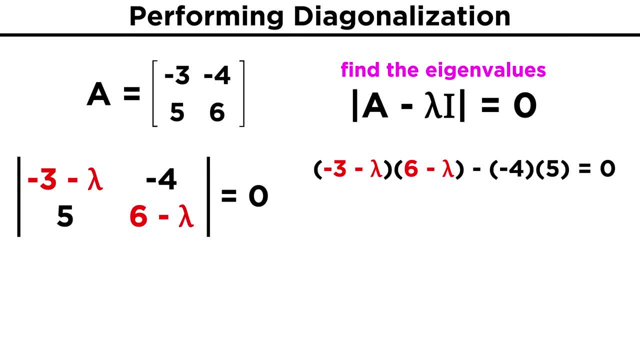 Taking this determinant, we get negative three minus lambda times six minus lambda. minus negative four times five equals zero. Foiling these binomials, we get negative eighteen plus three lambda minus six. lambda plus lambda squared plus twenty equals zero, which, when simplified, gives us lambda squared minus three. 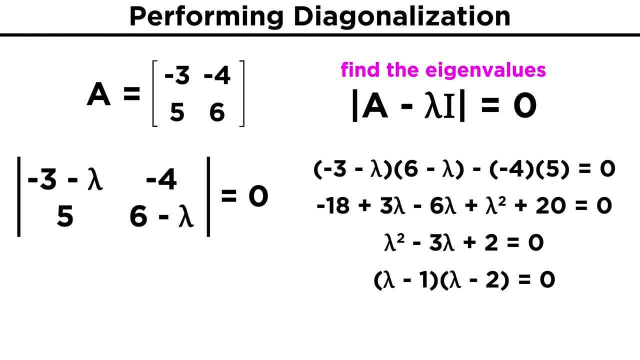 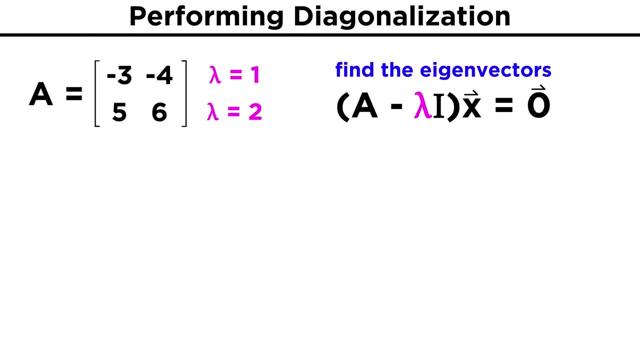 lambda plus two equals zero. Now, by factoring this, we see that lambda minus one times lambda minus two equals zero. This means our solutions and eigenvalues are lambda equals one and lambda equals two. Now to find the eigenvectors, we will plug in these values of lambda into the equation. 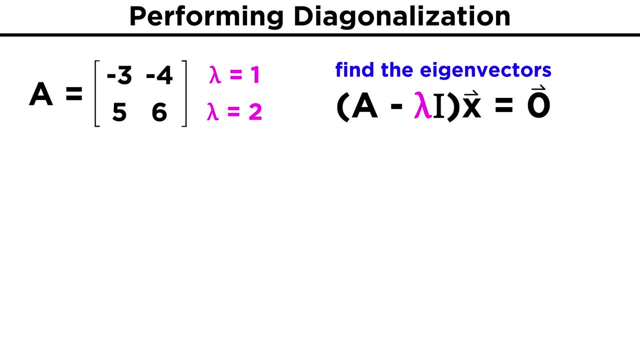 A minus lambda I, times X equals zero and solve for a possible vector, X, Starting with lambda, equals one. our matrix A minus lambda I becomes negative, four, negative, four, five, five. The top row ends up telling us that we have D. 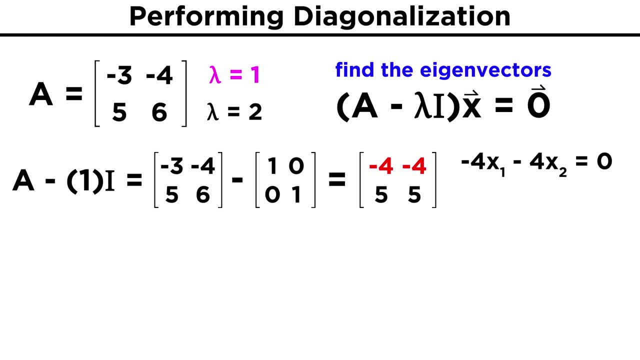 telling us that negative four X one minus four X two equals zero. Dividing by negative four, we get X one plus X two equals zero. or simply X one equals negative X two. We don't have to worry about the second row here, because it ends up giving us the. 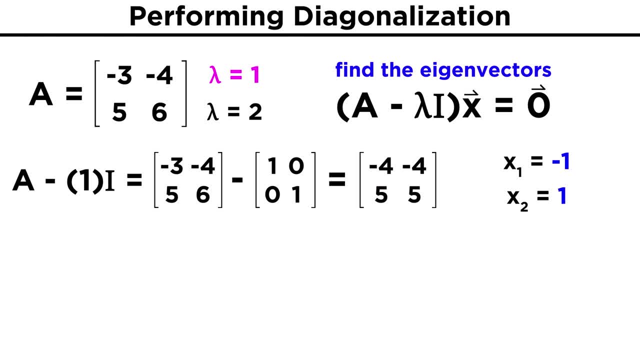 same thing. We will choose X two equals one, which means X one is equal to negative one. so our eigenvector for lambda equals one is negative one one. Now we will plug in lambda equals two. Our matrix A minus lambda I becomes negative five, negative four, five four. 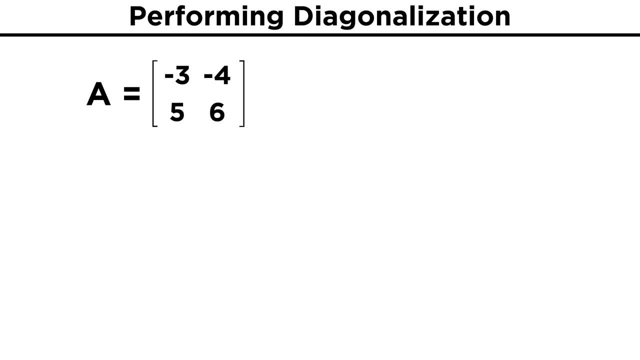 Consider the matrix A with entries negative three, negative four, five, six. We must first find the eigenvalues, which means we must solve for the values of lambda that satisfy this expression, where the determinant of A minus lambda I equals zero. Taking this determinant, we get negative three minus lambda times six minus lambda minus. 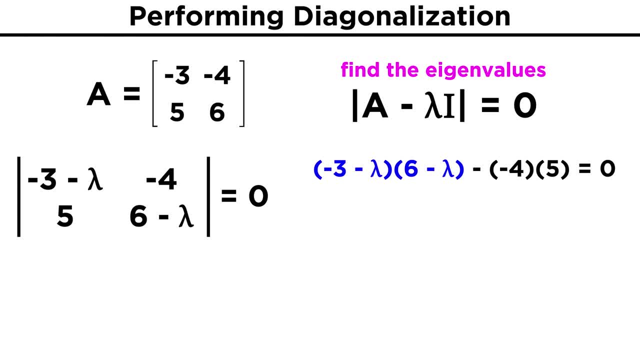 negative four times five equals zero. Foiling these binomials we get negative eighteen plus three. lambda minus six. lambda plus lambda squared plus twenty equals zero, which, when simplified, gives us lambda squared minus three. lambda plus two equals zero. Now, by factoring this, we see that lambda minus one times lambda minus two equals zero. 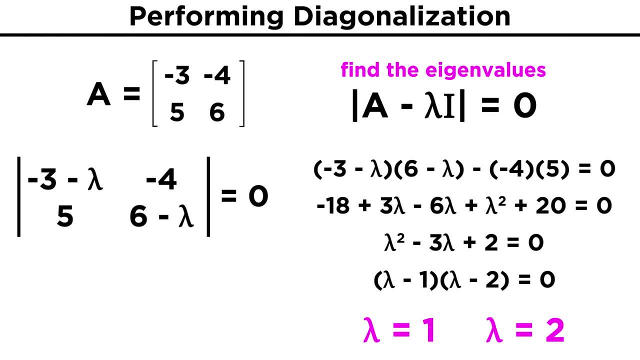 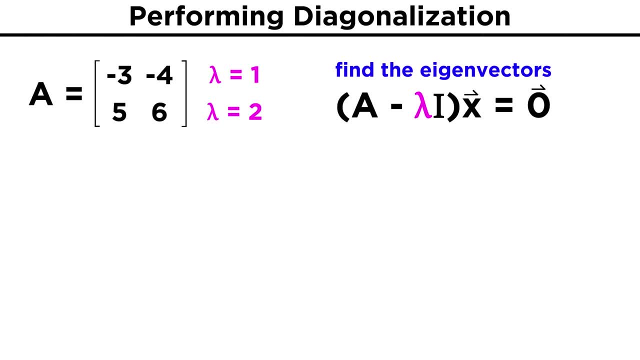 Which means our solutions and eigenvalues are lambda equals one and lambda equals two. Now to find the eigenvectors, we will plug in these values of lambda into the equation A minus lambda. I times X equals zero and solve for a possible vector X Starting with. 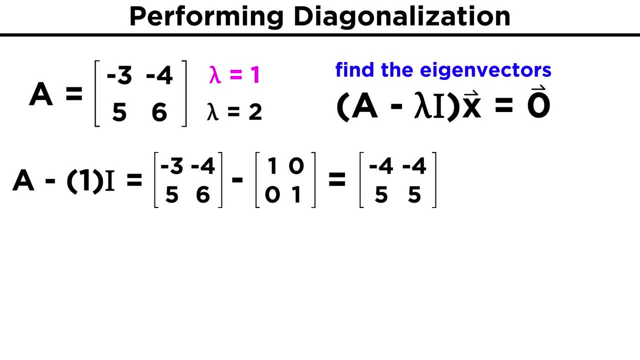 lambda equals one. our matrix A minus lambda I becomes negative four, negative four, five, five. This is telling us that negative four X one minus four X two equals zero. Dividing by negative four, we get X one plus X two equals zero, or simply X one equals. 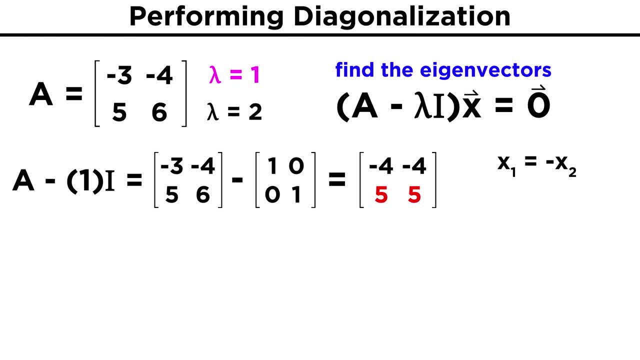 negative X two. We don't have to worry about the second row here, because it ends up giving us the same thing. We will choose X two equals one, which means X one is equal to negative one. so our eigenvector for lambda, equals one is negative one one. 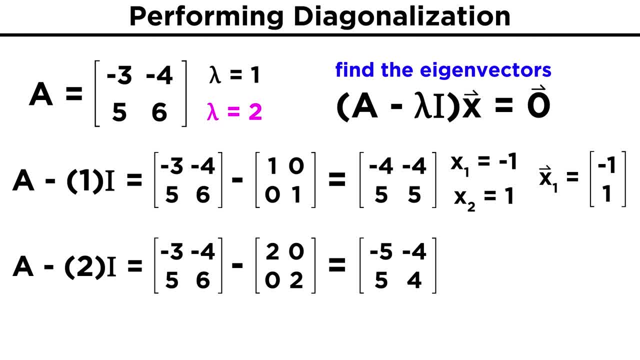 We will plug in: lambda equals two. Our matrix A minus lambda, I becomes negative five, negative four. five four. Both rows will again give the same result. but looking at the top row we get negative five X one minus four X two equals zero. 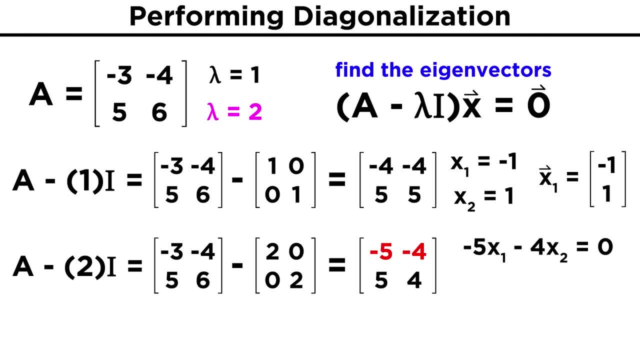 Both rows will again give the same result. but looking at the top row, we get negative five X one minus four X two equals zero. Solving for X one: we get X. one equals negative. four fifths: X two. Choosing X two equals one. we get X. one equals negative. four fifths. 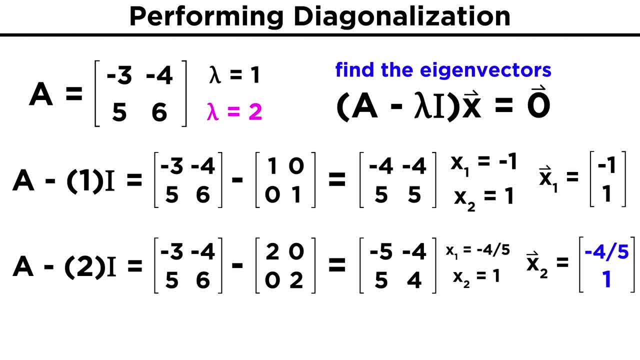 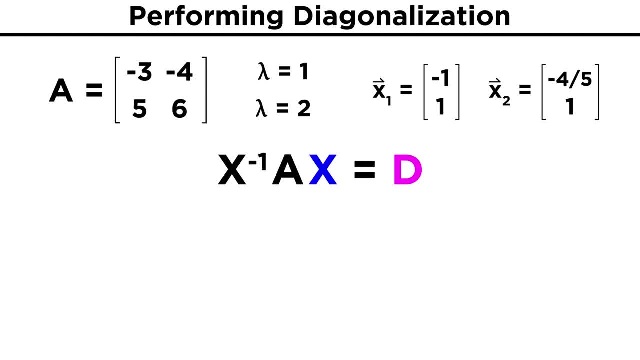 Using our eigenvector for lambda equals two. equal to negative: four fifths one. Now that we have all of our eigenvalues and eigenvectors, we can write out the diagonal matrix D and the matrix X. D will simply be the eigenvalues along the diagonal. D equals one. zero zero two. 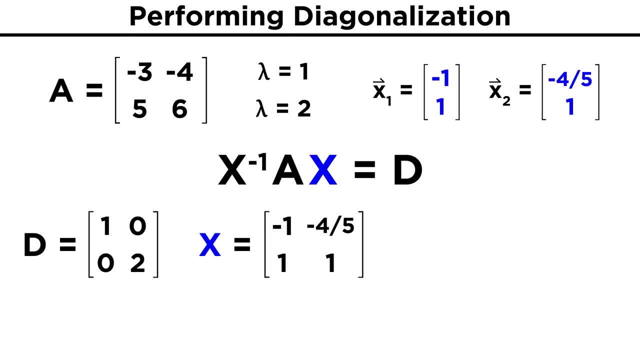 X will have the eigenvectors as columns, but now that we have chosen an order for the eigenvalues, we must keep that order in mind. The eigenvector for lambda equals one must be our first column, while the eigenvector for lambda equals two will be our second, making our matrix: X equal, negative, one negative. 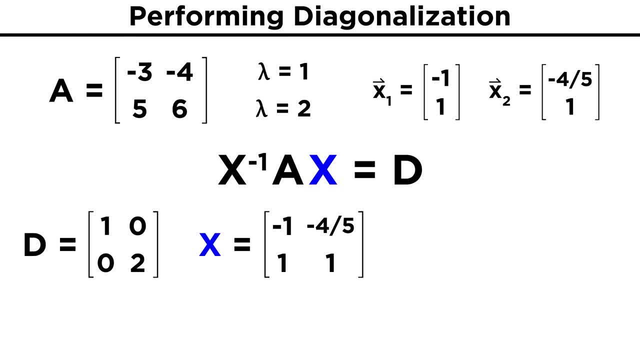 four fifths one one. We have obtained the main matrices for diagonalizing the matrix A. The only remaining piece is the inverse of X. Since X is a two by two matrix, we can write out the diagonal matrix D In a two by two matrix. we simply swap the top left and bottom right elements multiply. 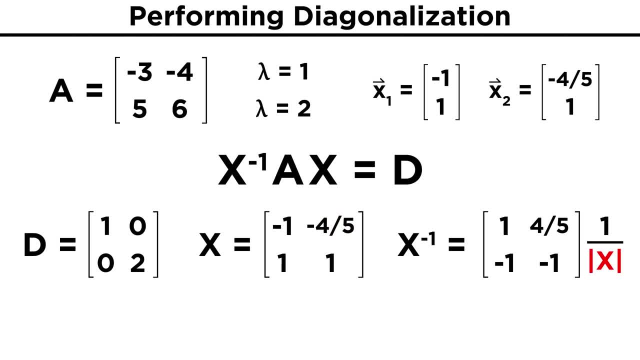 the off-diagonal elements by negative one and divide the whole matrix by the determinant. The determinant will be negative one times one minus negative four fifths times one which is negative one plus four fifths, which equals negative one fifth. The inverse will therefore be the matrix one, four fifths negative one negative one divided. 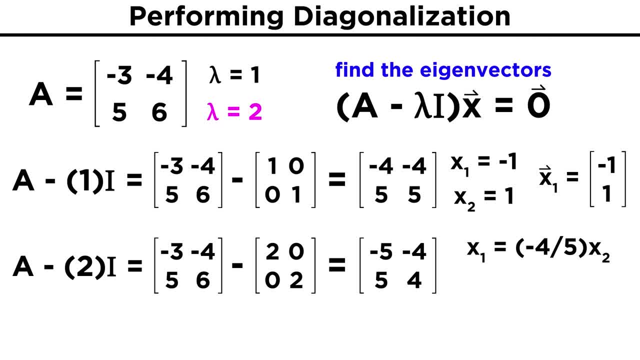 Solving for X: one, we get X. one equals negative four fifths X two. Choosing X two equals one. we get X. one equals negative four fifths. Making our eigenvector for lambda equals two equal to negative four fifths one. 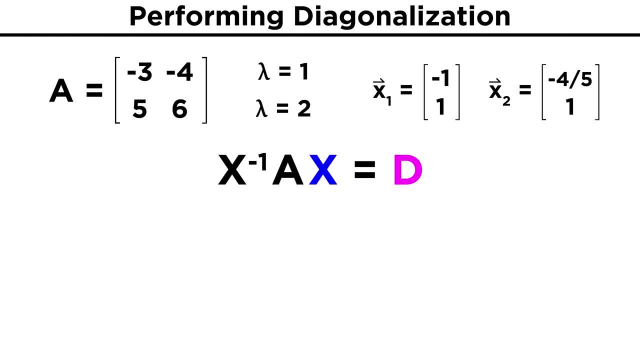 Now that we have all of our eigenvalues and eigenvectors, we can write out the diagonal matrix D and the matrix X. D will simply be the eigenvalues along the diagonal. D equals one zero, zero two. X will have the eigenvectors as columns, but now that we have chosen an order for the eigenvalues, 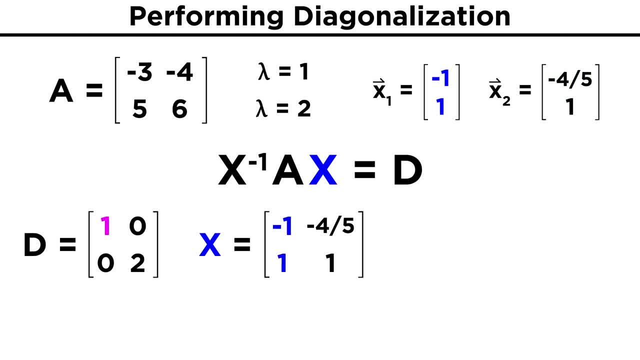 D equals one zero, zero, two values. we must keep that order in mind. The eigenvector for lambda equals one must be our first column, while the eigenvector for lambda equals two will be our second, making our matrix X equal. 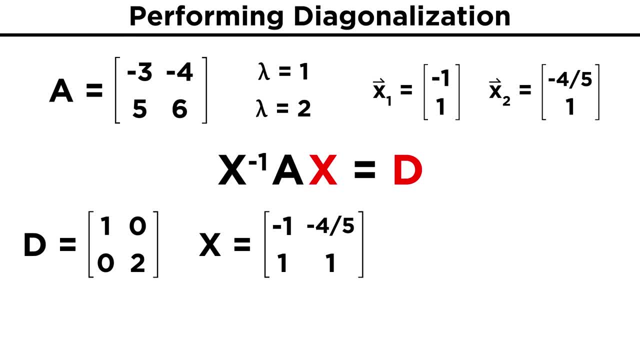 We have obtained the main matrices for diagonalizing the matrix A. The only remaining piece is the inverse of X. Since X is a two by two matrix, we simply swap the top, left and bottom right elements, multiply the off-diagonal elements by negative one and divide the whole matrix by the determinant. 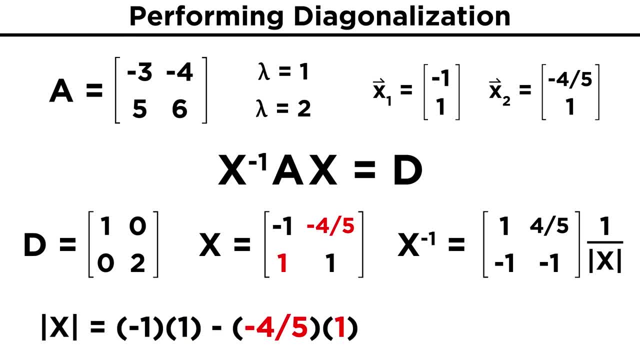 The determinant will be negative one times one, minus negative four fifths times one, which is negative. one plus four fifths, which equals negative one fifth. The inverse will therefore be the matrix one, four fifths. negative one, negative one divided. 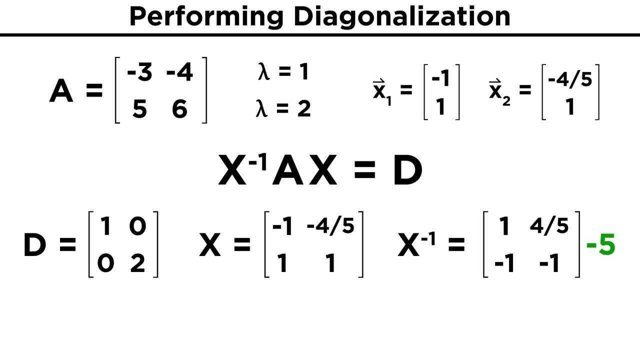 by the determinant, The determinant negative one. fifth, which means we just multiply by negative five, giving us negative five, negative four, five, five. We have found all the components to diagonalize A, those being X, D and the inverse of X. 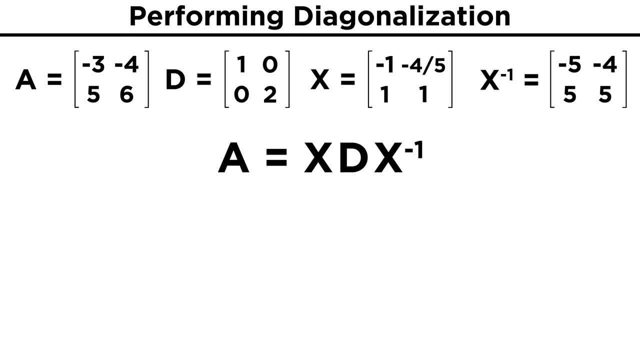 But in order to show that setting up the matrices in this way does in fact give back A, following the equation A equals X, D, X inverse, let's do the multiplication to verify First. take D times X inverse and we get negative five, negative four, ten ten. 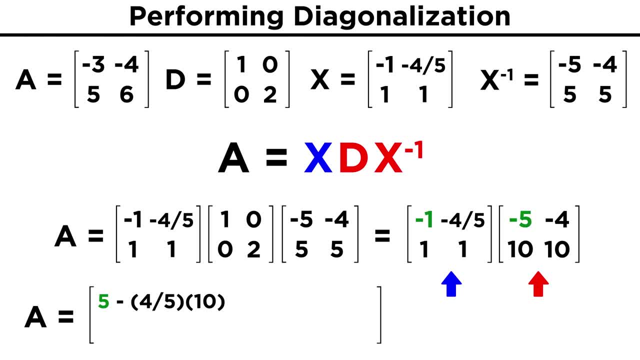 Next we will multiply X by this new matrix, giving us five minus four, fifths times ten. four minus four, fifths times ten. negative: five plus ten. negative four plus ten. This becomes five minus eight. four minus eight. five six. 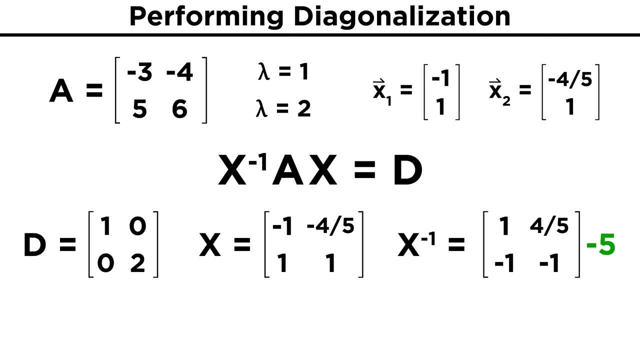 by the determinant negative one. We have found all the components to diagonalize A, those being X, D and the inverse of X, But in order to show that setting up the matrices in this way does in fact give back A following. 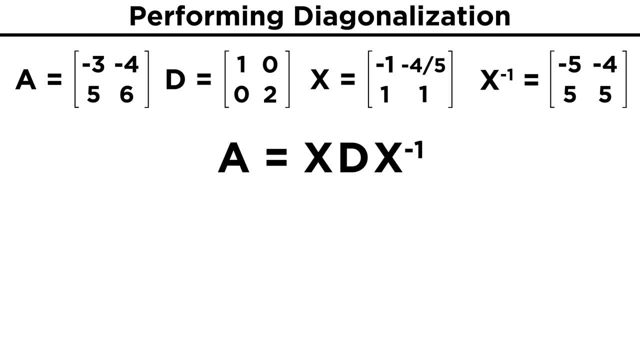 the equation: A equals X, D, X inverse. let's do the multiplication to verify First. let's do the multiplication. Let's do the multiplication First. take D times X inverse, and we get negative five, negative four, ten ten.